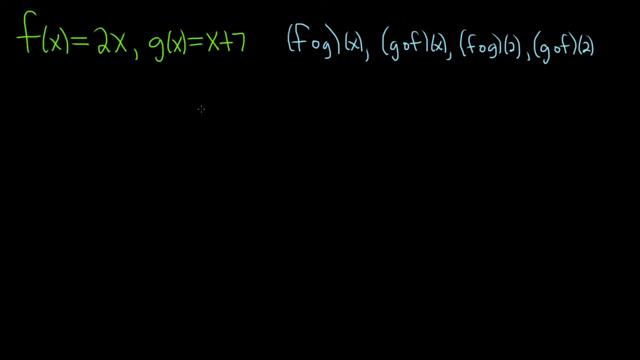 In this problem we have to compute various different things. So we have f of x equals 2 of x and g of x equals x plus 7.. The first part wants us to find f og of x. Let's go ahead and work through that. So when you have f og of x, so this is the same thing as saying f of and then g of x. 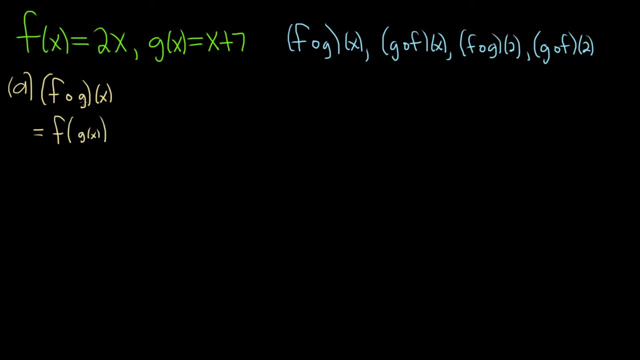 Okay, so it's written just the way it's written here. So you want to work from the inside out. So first you replace the g, So g of x here is x plus 7.. So you write down the f again, you write down the parentheses and then you just replace g of x with x plus 7.. 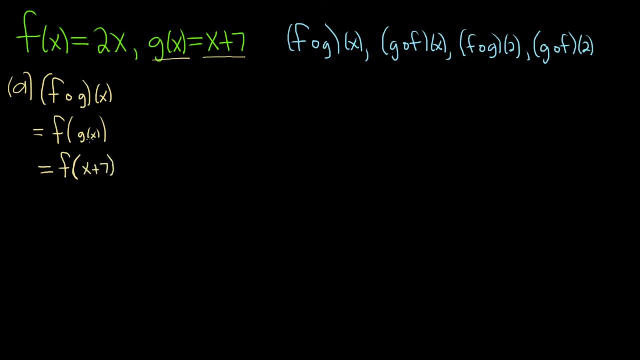 That's the first step And, again, it's pretty easy to memorize what it means because, look, it's f, g, f, g, It's in the same order. Okay, Then you look at f of x, because this is f, This is f of x plus 7.. Well, f of x is just 2 times x. 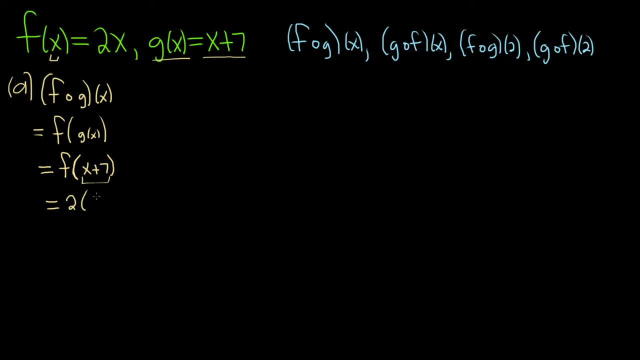 So f of x plus 7 is just going to be 2 times x plus 7.. So this basically means you replace x with x plus 7.. So you would get here- I'll do it up here, so you see it: x plus 7.. Just replacing. 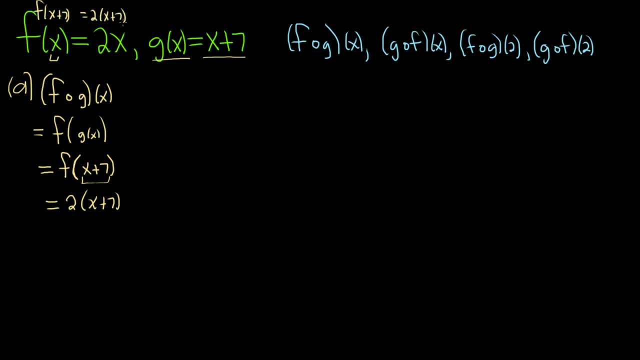 it, you get 2 times x plus 7.. That's all you do, And then just distribute So we get 2x plus 7. Plus 14.. So that would be the answer to the first part. Part B: very, very similar. So for part B. 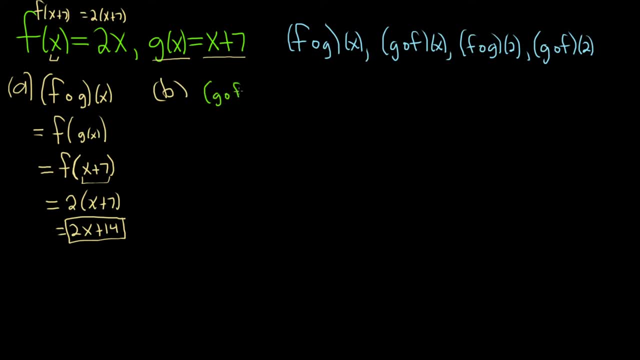 we just have to find g of f of x. So same thing as before it appears. it was written in the way it appears, So it's g of f of x, You see. so it's g, f, g, f, And then you replace the inside, So always. 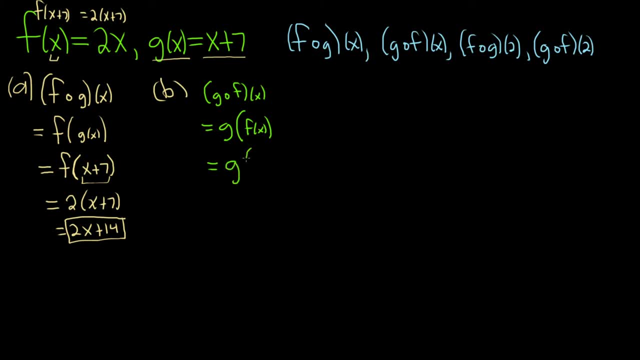 replace the inside first. So this is g of, and then the inside piece is f of x, So it's 2x. Just replace that, So 2x. And then now you look at g, because it's g of 2x. Well, g of x is x plus 7..